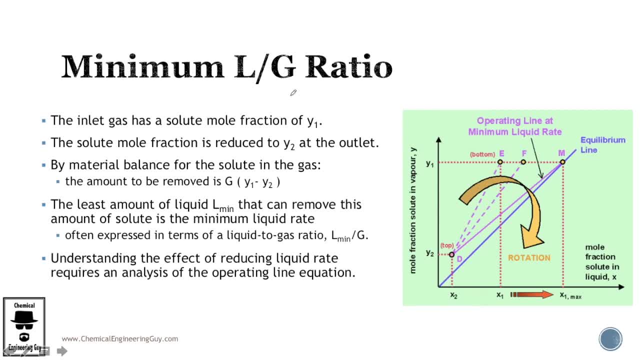 all right, all right. all right, let's talk about the minimum amount or ratio of liquid versus g or gas. remember that in engineering we're always interested in the mass transfer, but we're also interested in the material balance, so we don't want to spend that much of the solvent. 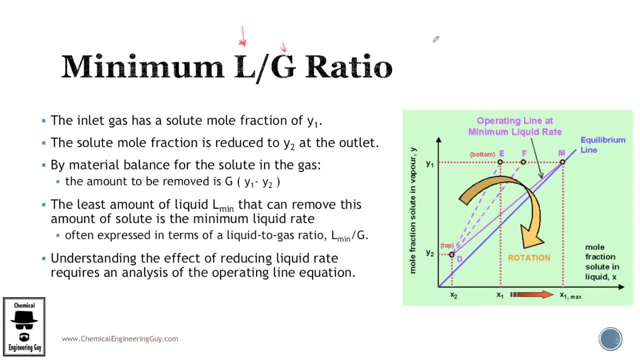 in order to clean this gas. now probably you're wondering: why not g? why are we focusing in l, the solvent? well, g is typically fixed because if you have your, let's say, you have a furnace here and you have a stack gas, this furnace is operating for maybe an electric generation. 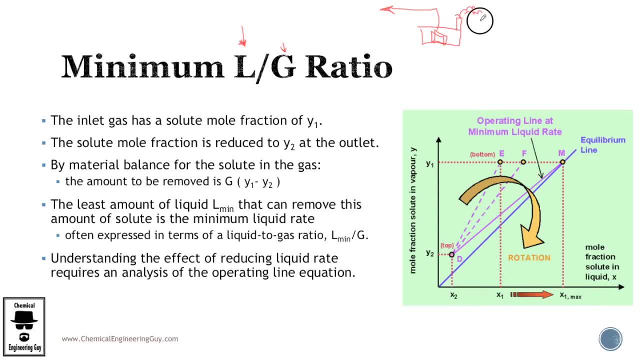 i don't know. let's say the process is fixed. they are producing this gas. let's call it g. well, g will be fixed, g is given and typically it's also given the percentage of the material that we want to clean. so if we are operating counter current, this will be. 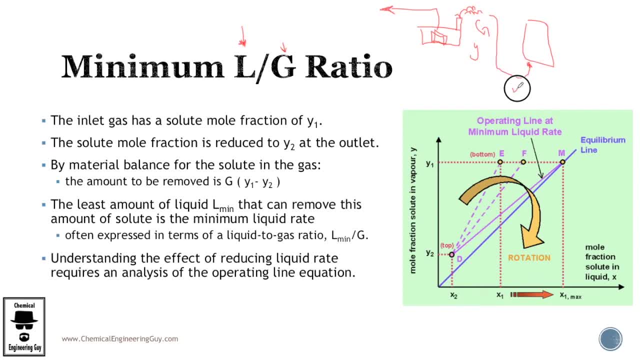 here, right going in the inlet of our absorber. this would be y1, let's say that this is three percent co, and we know that we need to clean this country currently with a liquid solvent which is expensive and this has a x2 value. so typically the x2 value, you know it because you choose the 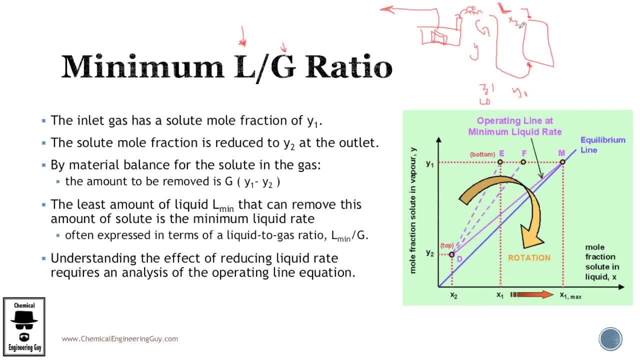 solvent, you select it. so x2 will be given. best case scenario, it's a zero percent. otherwise, well, try to prove this. what you know is that g is going to go out with a given specification. so this value, right here, guys, is also given or fixed. the government is telling. 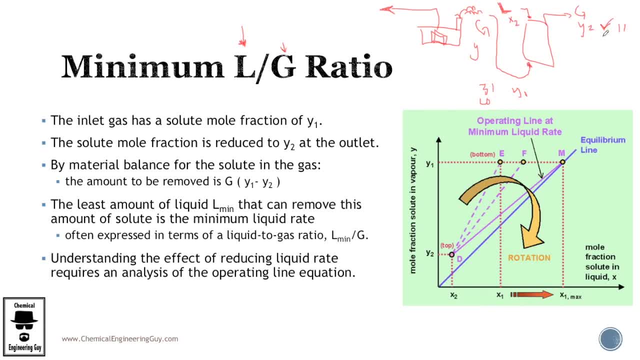 you that you need to decrease this to one percent. you should not change it. this will be your specification: one percent. so you have the inlet and the outlet of the gas. so g won't change. the gas is fixed. the solvent is the only thing that we can change if we add extra solvent. 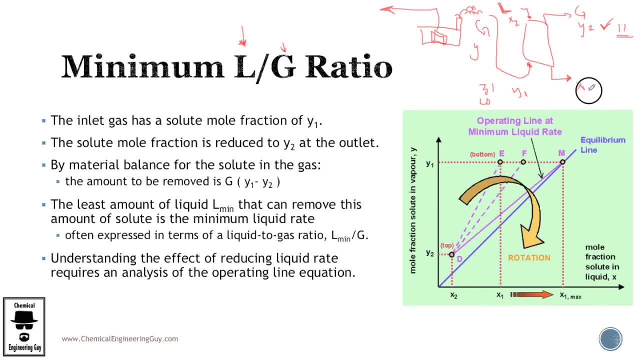 let's say: we don't care how much goes here, so let's say x1. what you want to do is to minimize the amount of liquid used. if you use too much liquid, that will be fine, we will achieve the point, but we are going to be throwing away solvent. so you want to see what will be the best case scenario. 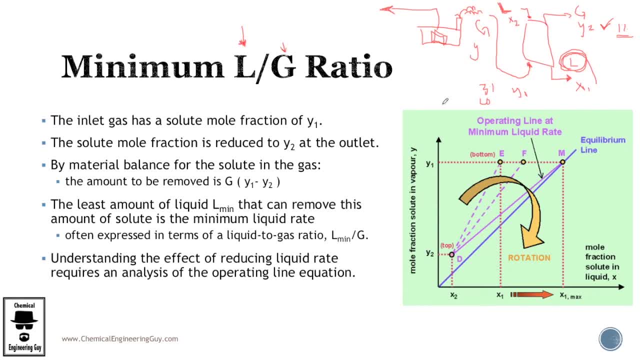 this is very typical for- oh, i like to compare this as with the karner cycle- that at least you have a standard in your engine and you know how much until you are perfect. super reliable, but also is the best case scenario typically 70% efficiency. 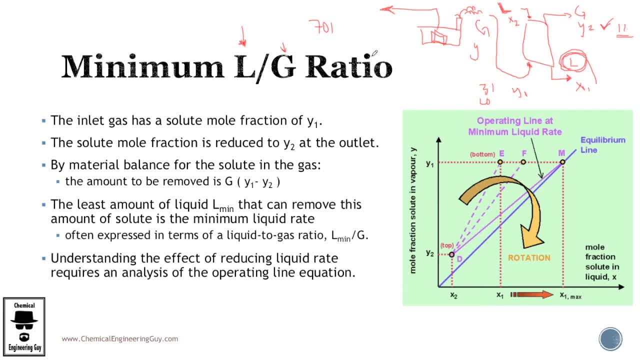 according to Carnot. you know that you will never, ever have a engine that goes above 70%. This is also true with the minimum LG ratio. you will see that the best case scenario given a G is the L value here. Okay, let me read this here: 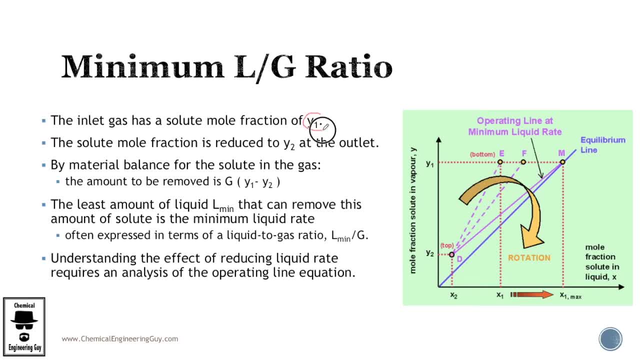 The inlet gas has a solute mole fraction of Y1.. Okay, so that's true. stated before, G will have a fixed value of Y1.. This is coming from the stack gas. you cannot change it. The solute mole fraction is reduced to Y2 in the outlet. 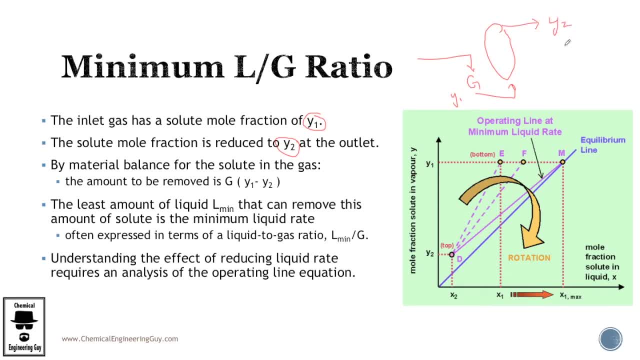 Stated before, guys, there is a value, environmental value, or maybe you need to clean this for the following process, for your machines, equipment et cetera. this will be also a specification, Given the material balance if you were to make. 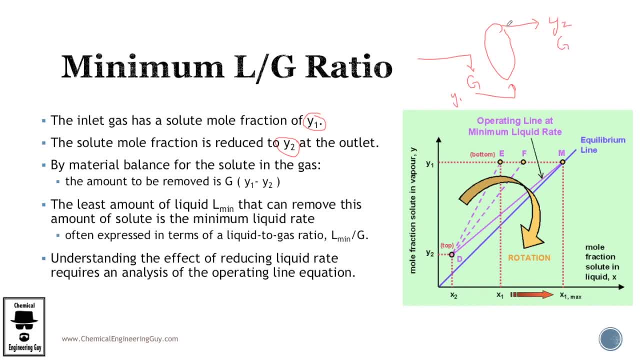 a material balance, you will see that the actual amount of solvent- sorry, of solute- is not disappearing. it's going to L. But if you want to check that, simply make a balance on G. You will have this, The least amount of liquid required to remove this amount. 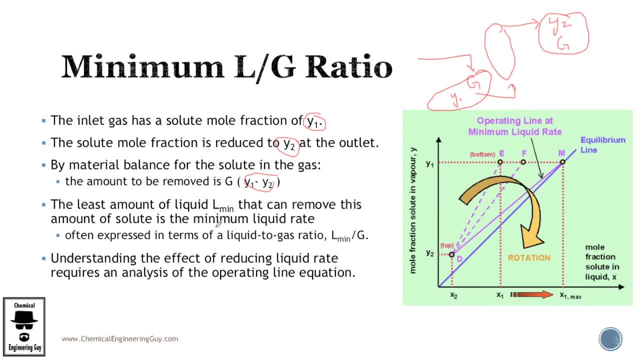 is called the minimum liquid rate, L minimum. Typically in the industry what we do in absorption is to calculate the amount of liquid we will give the liquid to gas ratio, the L mean divided by G Stated before this one right here. 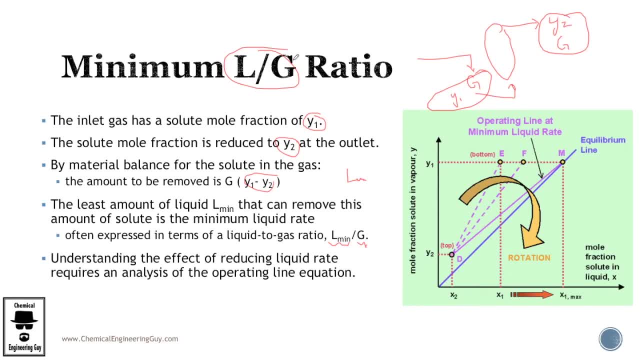 Why? Because it's normal to do so and it will never depend on G. This is based on G, so if you were using 100 amounts of G, you just need to multiply this amount by 100.. If you were using five, you just need to multiply this. 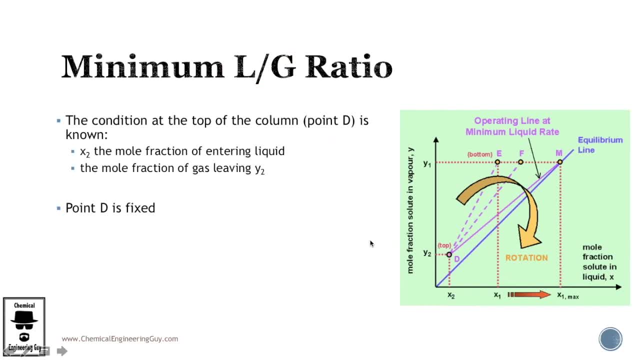 by five and so on. Okay, continue The condition at the top of the column, point D, which is this one right here Is known why? Because we select X2, and the gas must be given at Y2.. 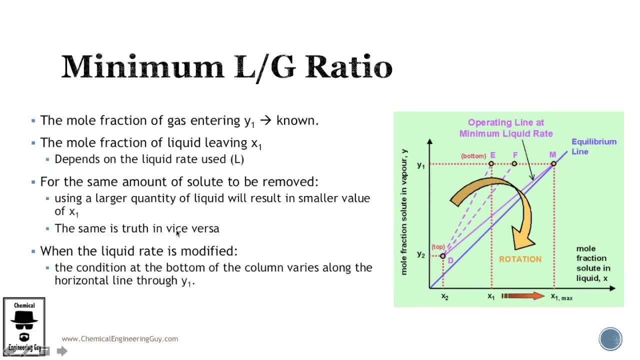 So the point D is fixed. The mole fraction of gas entering is known. It's actually the stack gas. The mole fraction of liquid leaving depends on the amount of liquid rate. So this is interesting- Now we're talking about that- depending on the amount of L that we use. 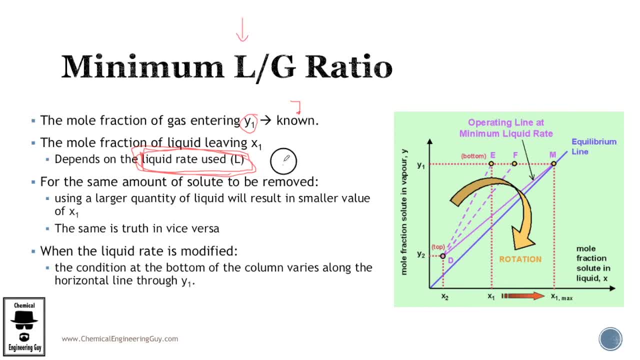 X is fixed or X1 is fixed. So if you have high value of liquid, you're going to have a low value of X1.. You have a very low value of L, you're going to have the higher amount of X. 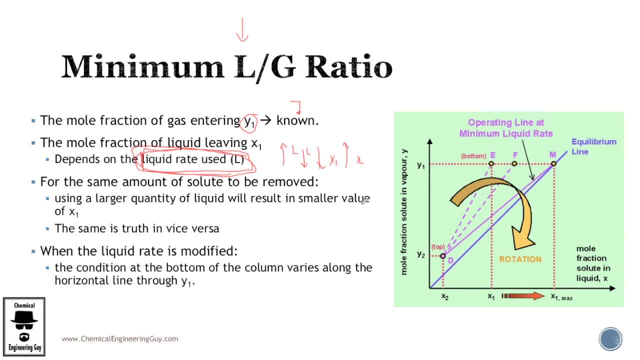 For the same amount removed. using a larger quantity of liquid will result in a smaller amount of X, and the same is true vice versa. It's exactly this what I explained you. When the liquid rate is modified, the condition at the bottom of the column varies along the 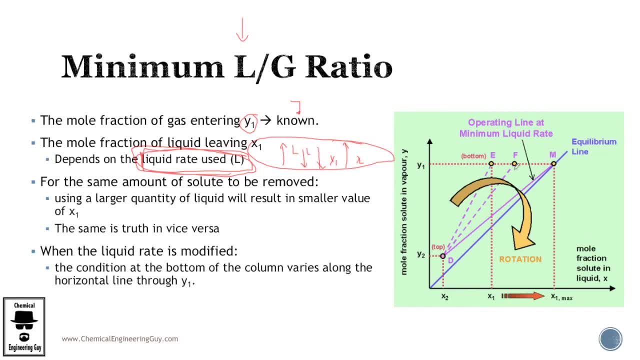 horizontal line through Y1.. Okay, So this is interesting. This is Y1.. So that's why we've got these several points. X1 can move from left to right up to a maximum amount. Hopefully you get the idea which one is the maximum. 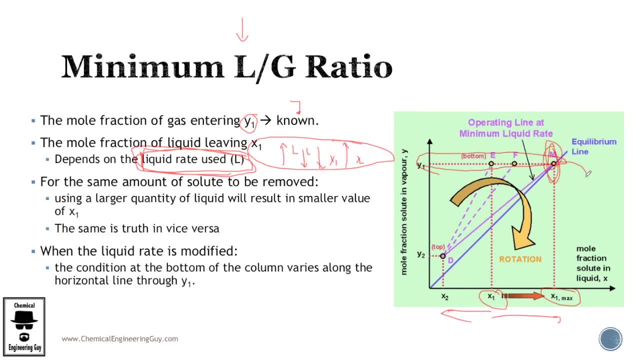 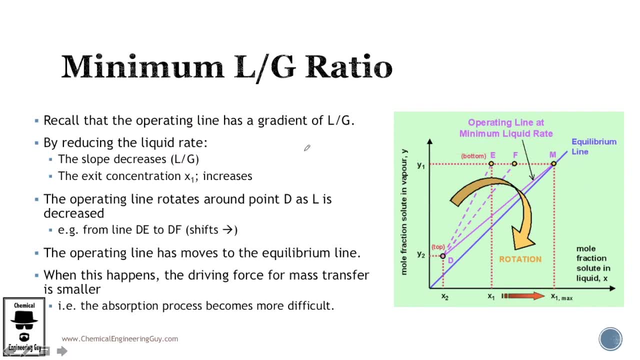 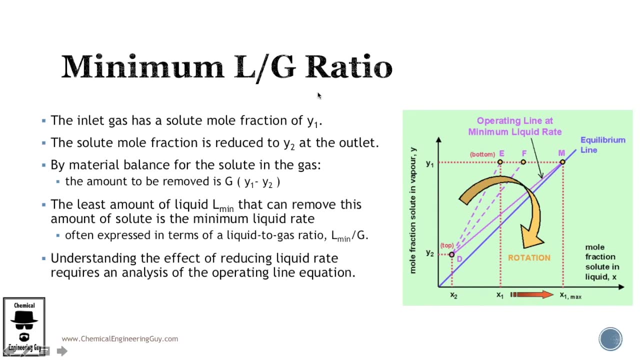 Yeah, The equilibrium line. You can never go away. If you're observing, you will never go backwards. Recall that the operation line has a gradient or a slope of L divided by G, which that is maybe the reason that we use this in the industry gas. 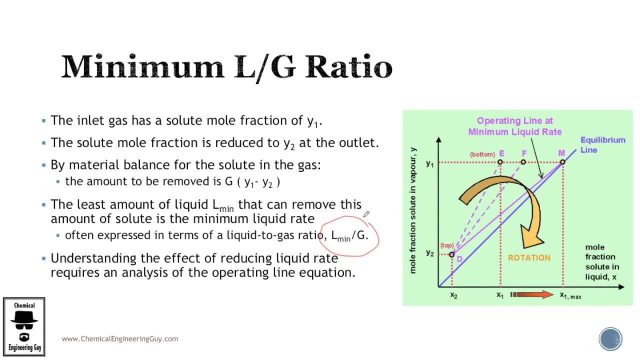 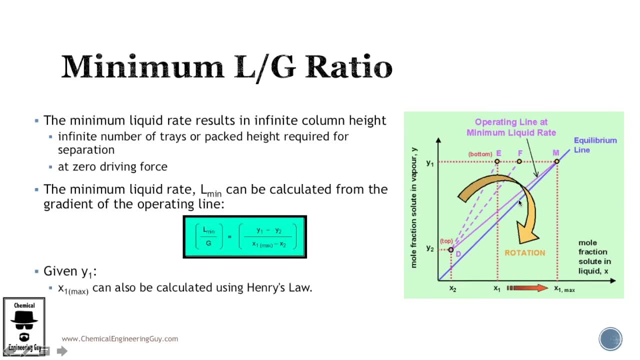 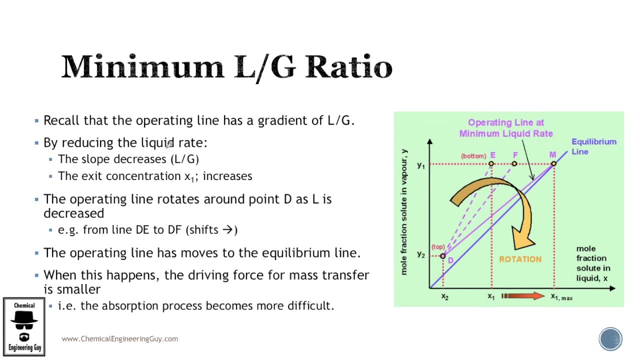 Remember. Yeah, It's because it is not only convenient, it appears graphically here. So this is L divided by G. Wait for it Here. By reducing the liquid rate, the slope decreases. So, as you can see, there is a shift to the right. 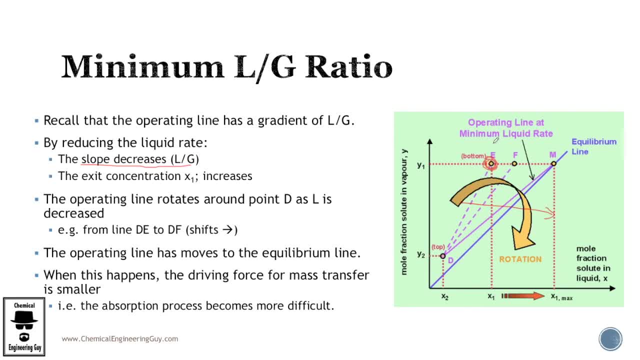 When we use a lot of L or solvent or liquid, you got point E Okay. When you start decreasing, you move to F. When you actually decrease to the best case scenario, you will get this amount here. If you were to use less amount of L, you will not be able to achieve the Y1 value. 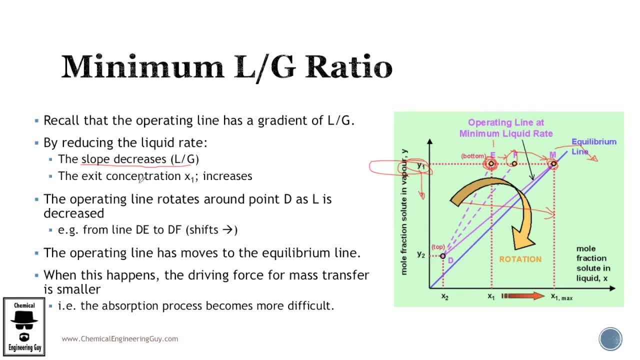 You will have maybe a value lower than here. The exit concentration X1, increases. So let me clean this up. You can see how, for E, we have a low value And as we approach M, We are increasing X. Hopefully you get the idea. 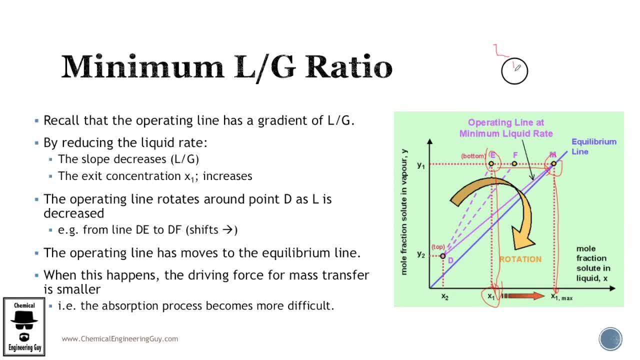 Because if we are using less solvent, then the solvent must be more contaminated with our solvent. If we are using a lot of solvent, we are going to dilute a lot of pollutant or solute in here, So that's why your X amount will be lower. 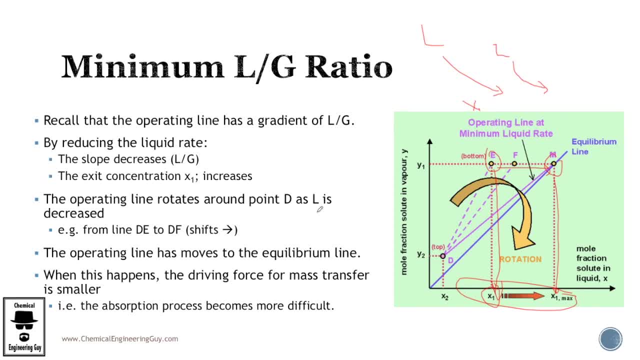 The operating length rotates around point D as L is decreased. That's what I'm telling you. Actually, I hate the word rotating, I love more like shifting. You can see that. You can see how it is going to the right. The operating line has moved to the equilibrium line, which is the top of the line. 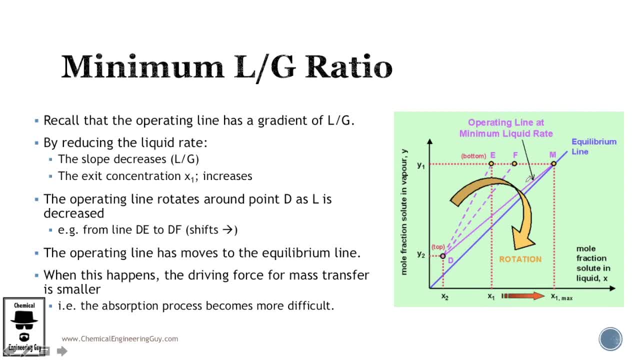 Now, interesting fact: right here, guys, As you move L to the right, you will see that the driving force. remember that driving force is always the line versus the point. So here to here we have a driving force, Here to here we have other driving force. 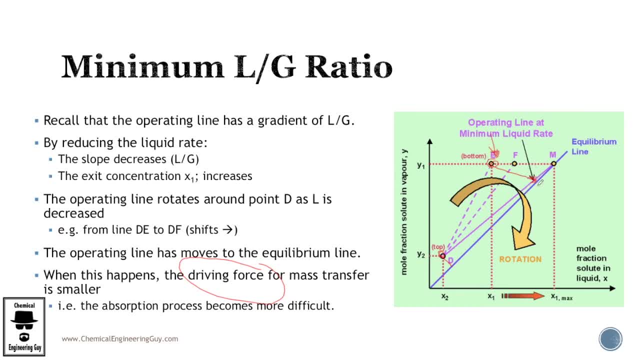 So when we use a lot of liquid, we are having a lot of driving force. When we are using the M value, we are technically with no driving force. So that's how our absorption process will become. If we are using E, it will be easily, but we are going to spend a lot of money. 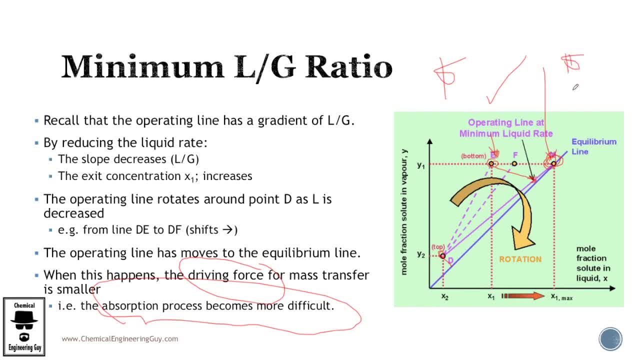 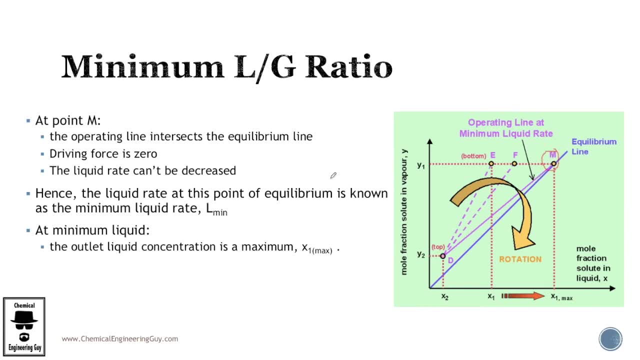 If we are near M it's going to be cheaper, but it's going to be hard to achieve. A little notes on M: The operating line intersects here, So you can see our operating line was first here, Then we're shifting here. 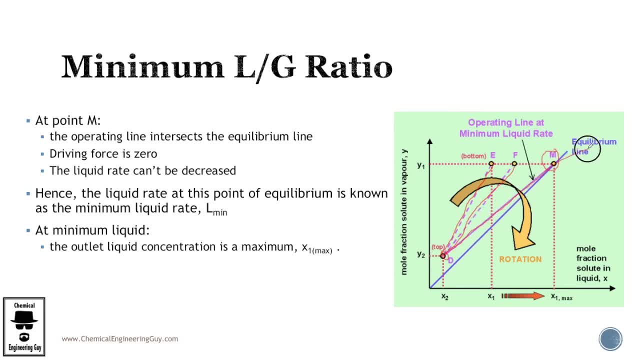 Until, eventually, we're forcing our operating line to cross, And this point right here, in which we cross, it is the value M. The liquid rate can be decreased, Actually, you can decrease it. What you're going to do is decrease this value, right here. 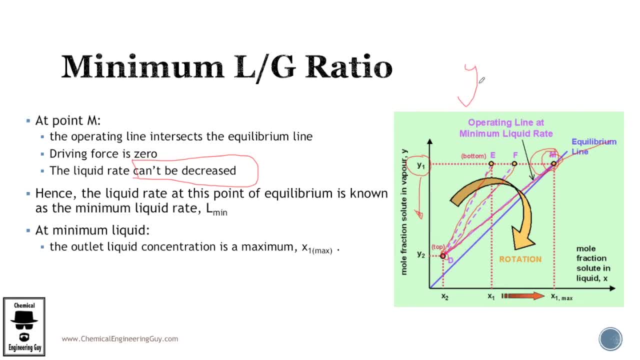 Which, of course, is not valid, because you are going to increase the content of- Let's see how it- Let's say the amount of percentage of gas going off. So in the previous example, if you have 7% maximum amount of CO, 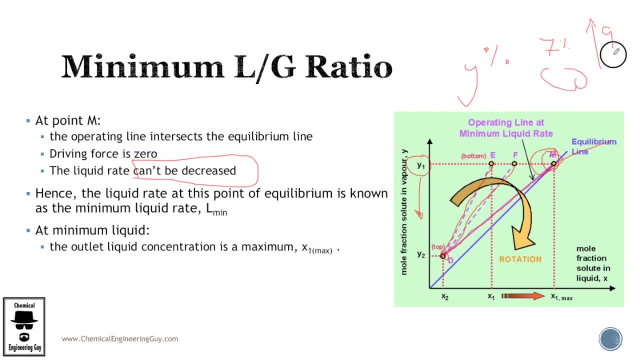 what's going to happen is that you're not going to achieve that. You're going to achieve 9%, 12% and so on. Hence the liquid rate at this point of the equilibrium is known as the minimum liquid rate. So if you were to get the L value here, 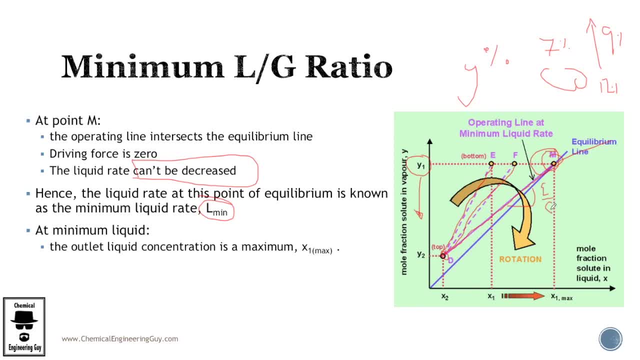 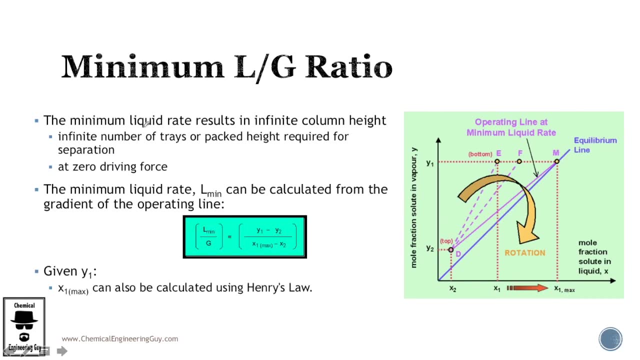 remember that the slope is L divided by G. If you know G, you can get L from the slope. And at the minimum liquid, the outlet liquid concentration is X1 max. This one right here, The minimum liquid. Okay, Okay, this is an interesting fact. 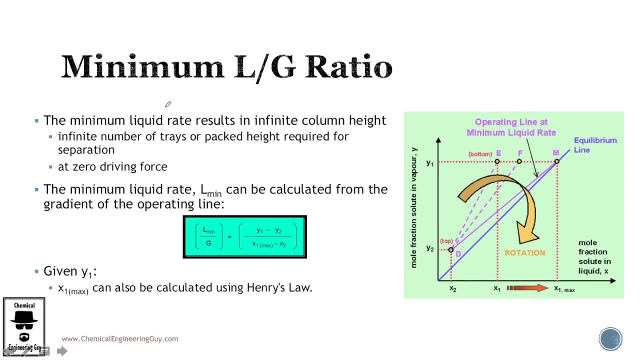 Right now we're not analyzing heights, But just to remind you, whenever you want to achieve equilibrium, technically it's impossible, or at least you need an infinite process. Therefore, if you were to model this absorption column and you want to achieve here, 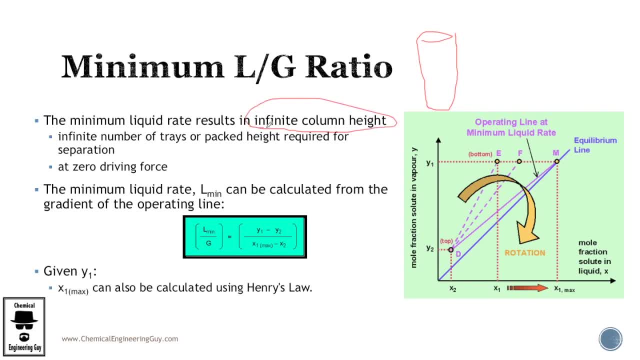 you will require an infinite column height. It's like exponential. You will see that eventually it goes, goes, goes and it keeps going and going and going and the asymptote value is a Cleveland line Zero driving force. You cannot divide by zero. 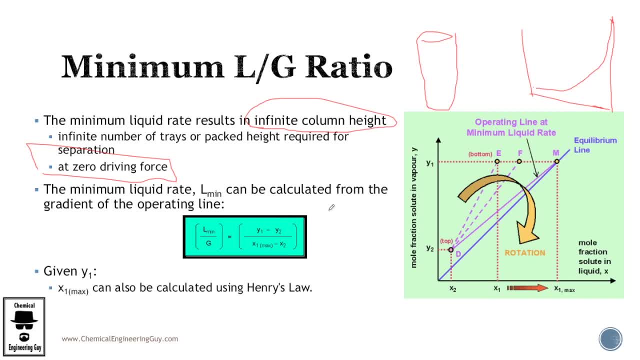 The minimum liquid rate. then, Guys, hopefully you remember the equations. The equation is not changing. The only thing that changes is that if we want to set up the minimum amount here, you need to set up the minimum amount here. Now, this is fixed. 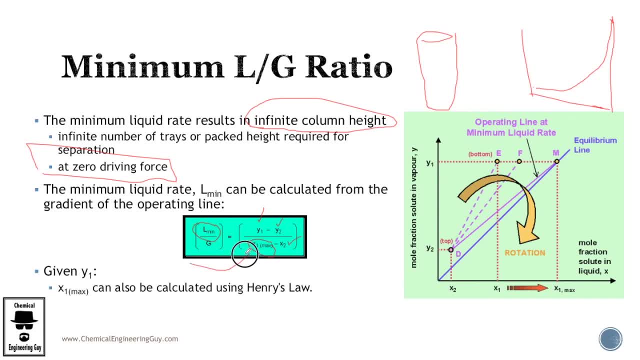 This is fixed. This is fixed And this must be calculated. Now hopefully you get to saw the Henry's law video because we will see that x can be calculated from Henry's law. If you have y and x Henry's law, you have Henry's constant. 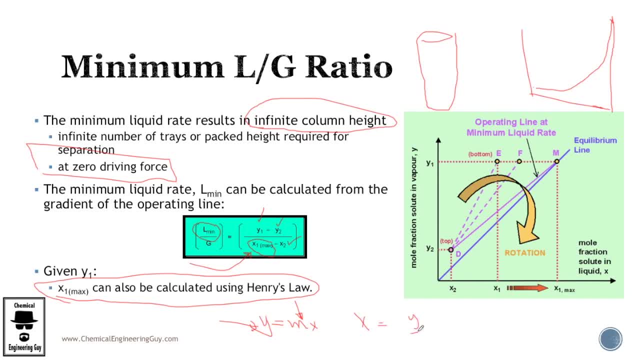 And if you have y, then you just solve for x, which will be this: You're talking about 3% divided by the Henry's constant, and you got your x value. Okay, a little bit more math. Remember that for a straight line.